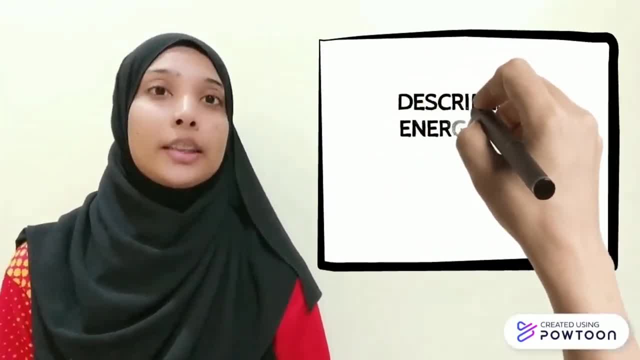 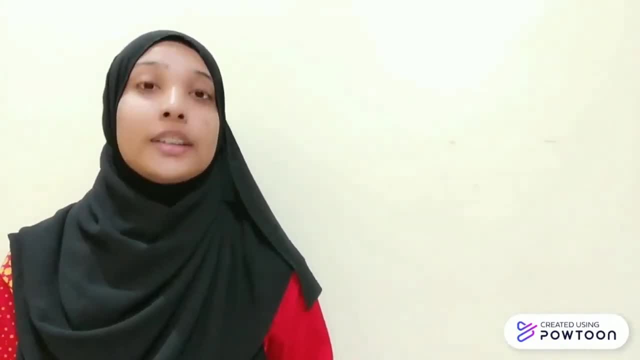 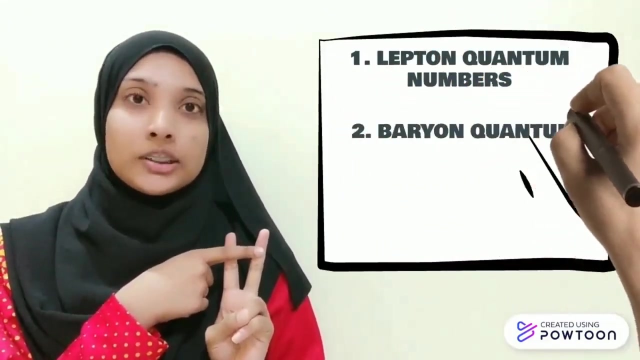 it describes the energies of electrons in atom because of that motion of an elementary particle or systems. When we are talking about interaction of elementary particles, those interactions happen in such a manner that we can associate a set of numbers, namely the leptin quantum numbers, the baryon quantum numbers and the strangeness quantum numbers. 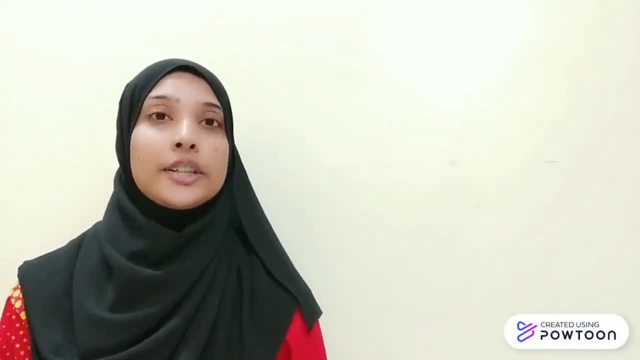 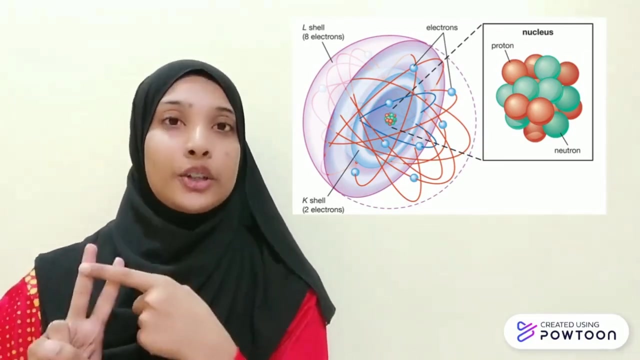 Next, in this video, we are going to discuss about quarks. Since we are a cave, we were told that all the stuff around us is made out of atoms. We know that atom is made out of protons, neutrons and electrons. Electrons are elementary particles. They are not made. 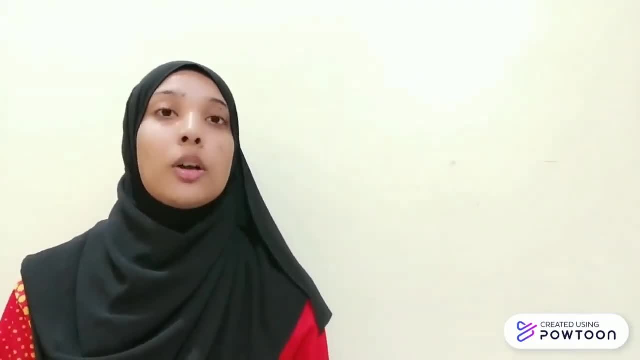 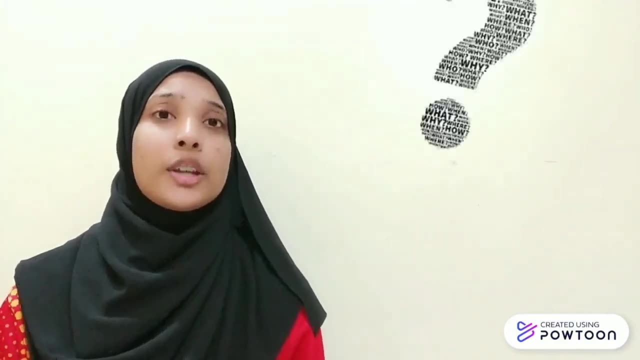 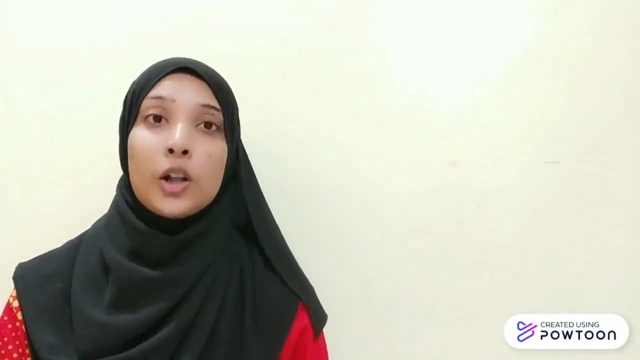 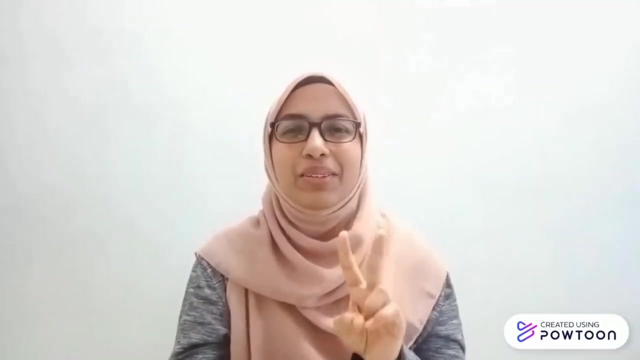 up of further fundamental particles. However, protons and neutrons are not elementary particles. Have you ever wondered what these protons and neutrons are made of? They are made out of two other fundamental things which are called as quarks. Now we are going to look at two types of quantum numbers, which are baryon numbers and 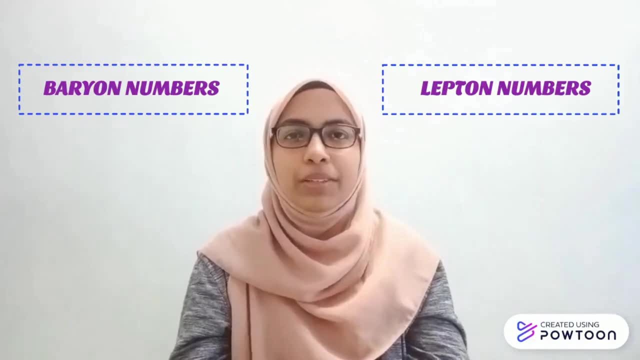 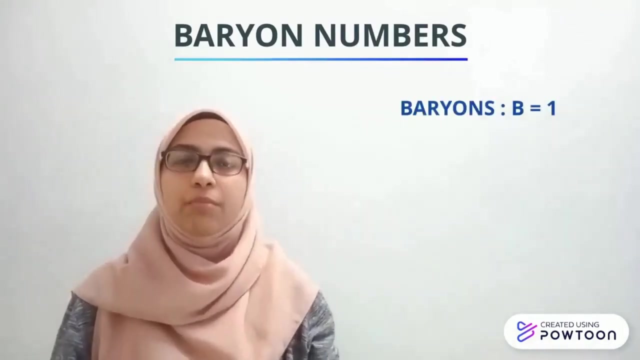 lepton numbers. Baryon and lepton numbers are properties possessed by all subatomic particles, which means that each particle has its own baryon and lepton number. Firstly, let's look at baryon numbers. All baryons have a baryon number of 1 because they are 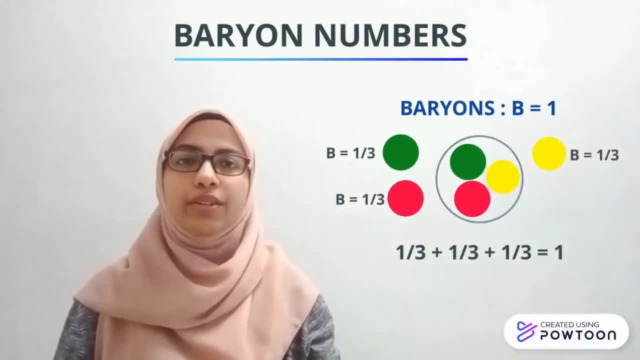 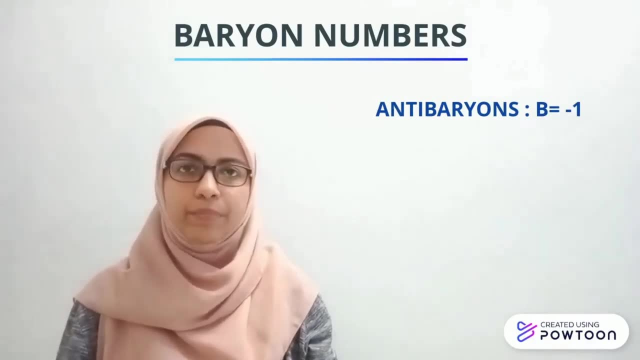 made up of three quarks and each quark has a baryon number of one third. So each quark has a baryon number of one third. This is similar to all antibaryons, which has a baryon number of negative one, because they are made up of three antiquarks with a baryon number. 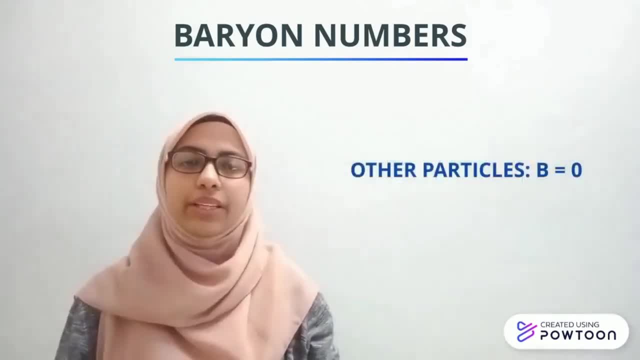 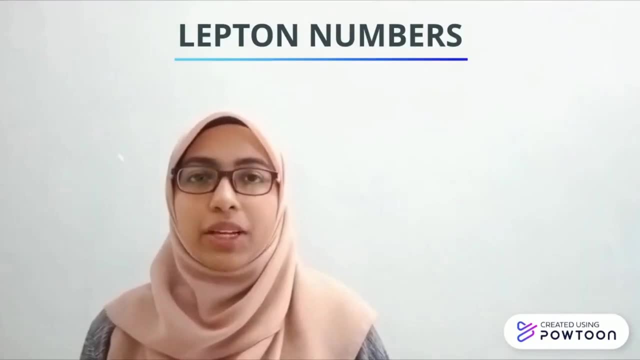 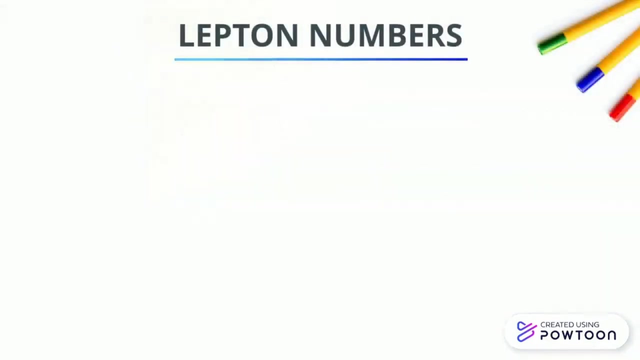 of negative, one third. All other particles have a baryon number of zero. Now we move on to lepton numbers. There are three types of lepton numbers, which are: electron lepton number, muon lepton number and tau lepton number. Here we can see that the lepton number 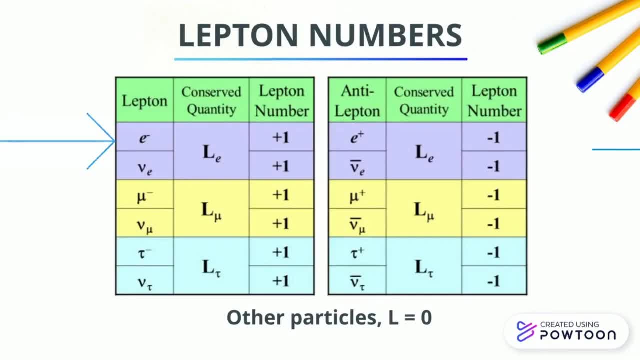 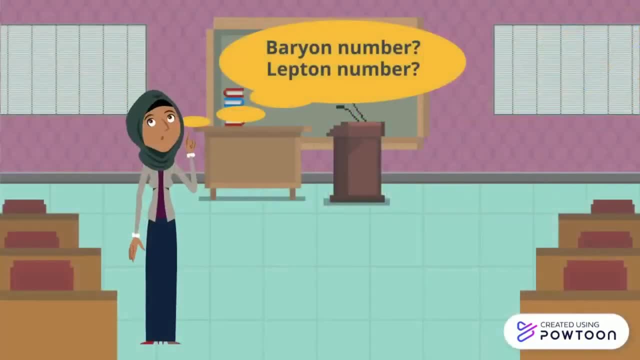 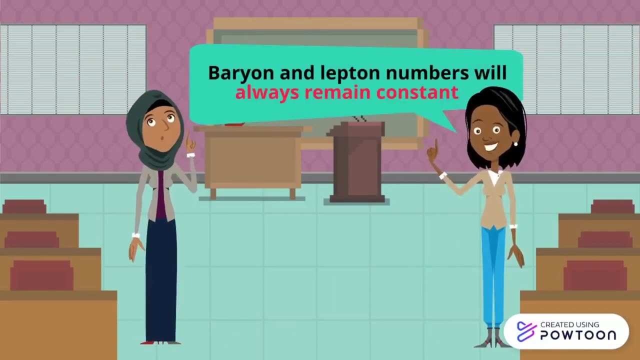 for each particle is positive one, For their antiparticles it is negative one, and all other particles have a lepton number of zero. You must be wondering what is the purpose of the baryon and lepton numbers. Actually, in each process that occurs in nature, the baryon and lepton numbers will always. 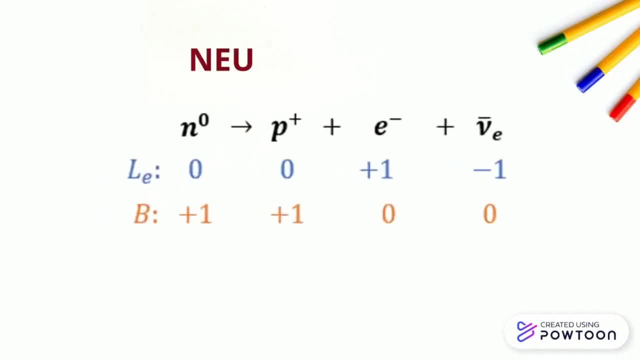 remain constant. For example, in the process of neutron decay we can see that the electron lepton number is zero both before and after the reaction. Similarly, with the baryon lepton number, it is positive one before and after the reaction. 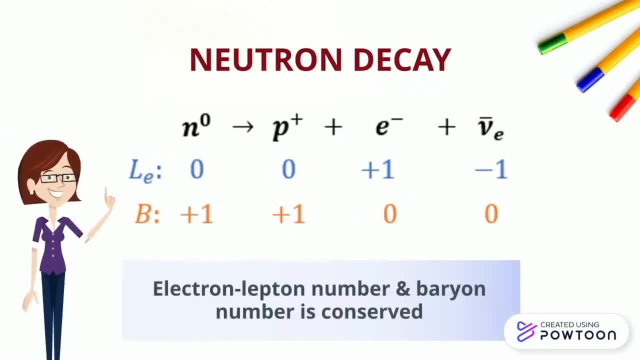 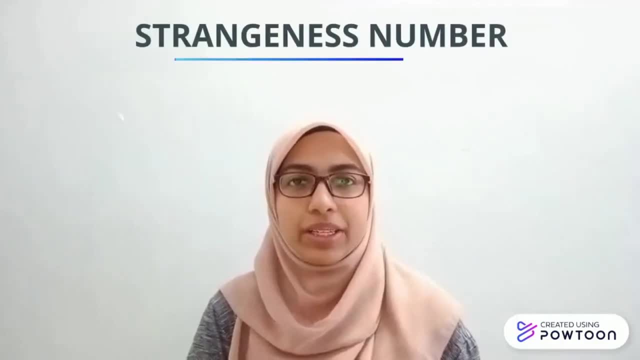 This means that the electron lepton number and the baryon number is conserved. Strangest number is a property of particle which depends on how many strange quarks or antiquarks they have. A strange quark has a strangest number of negative one and a strange 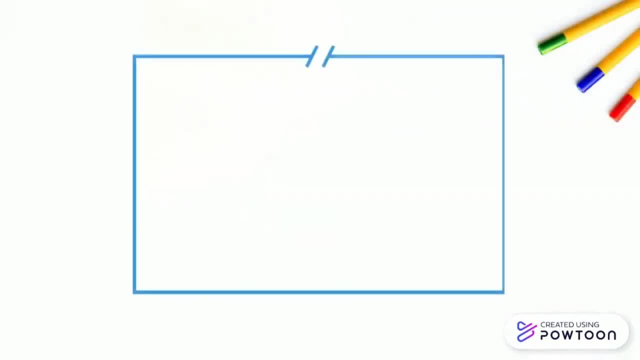 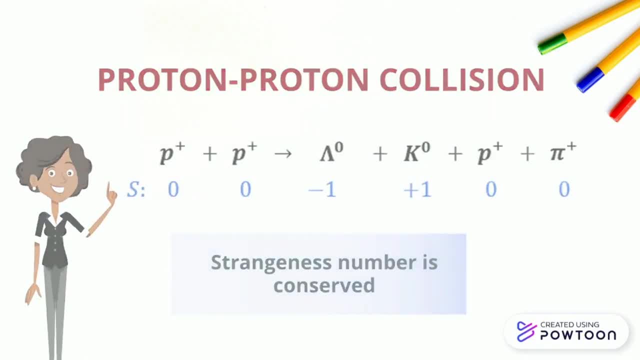 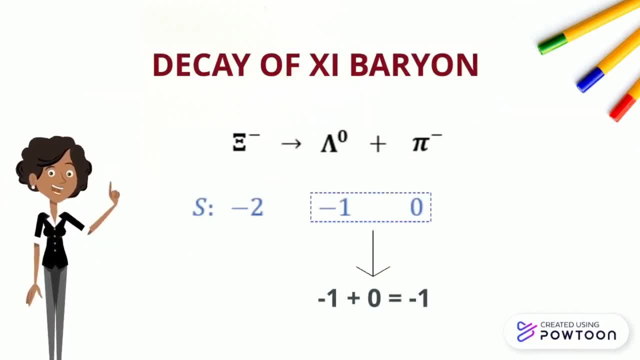 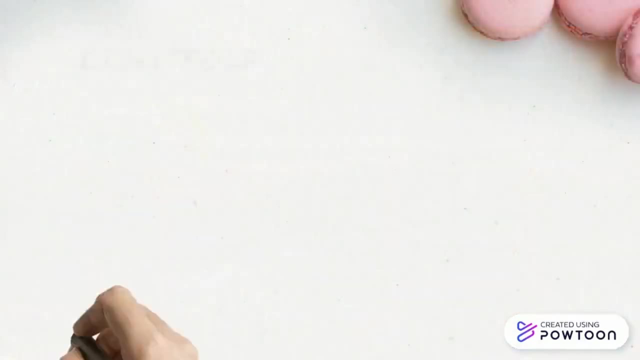 here in the decay of Zyberion, the strangest number before the reaction is negative 2, and after the reaction the total strangest number is negative 1,, which shows that the strangest number is not conserved. Eightfold way is a classification system of hadron into groups or geometric pattern based. 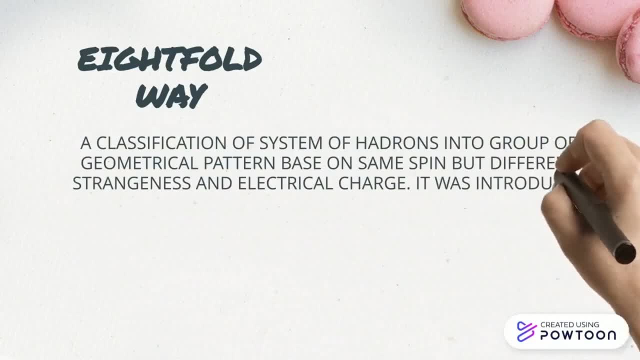 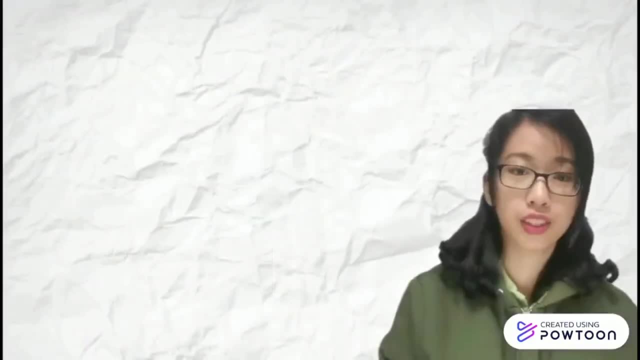 on the same spin but have different strangeness and electrical charge. It was introduced by Yuval Niemann and Muregelman. The first supermortiflate that they found was the Baryon Octet. Baryon Octet have eight. 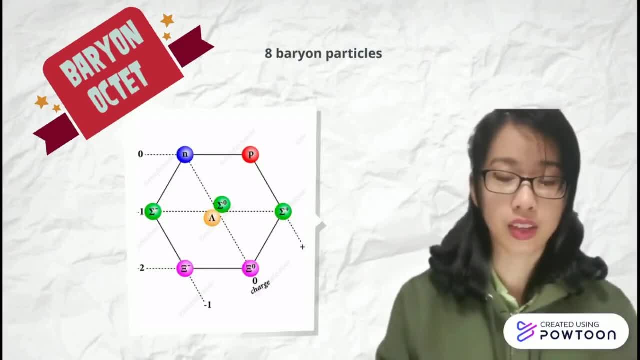 baryon particles which are arranged in a hexagonal pattern. All of these particles have the same spin, which is 1 over 2, but have different strangeness and electrical charges. For example, the proton and the neutron have the same spin. Baryon Octet have the same strangeness- quantum numbers of 0, but proton have the electrical charges of 1, while neutron has the electrical charges of 0.. Later on, Meson Octet was finally discovered. This supermortiflate consists of eight meson. 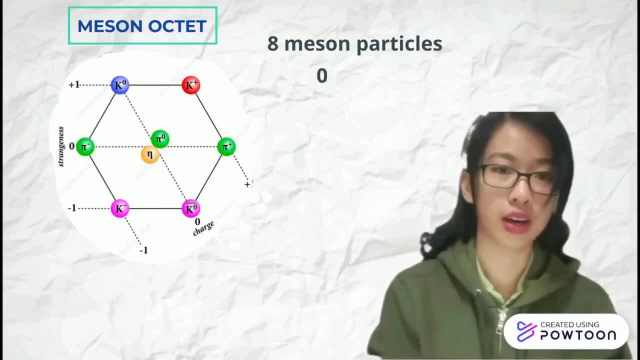 particles which have the same spin of 0.. This supermortiflate is different from the previous one as it has anti-quarks located on the opposite edge of the particles. For example, the positive kaon is located at the top right of the hexagonal pattern, while on the opposite edge it has. 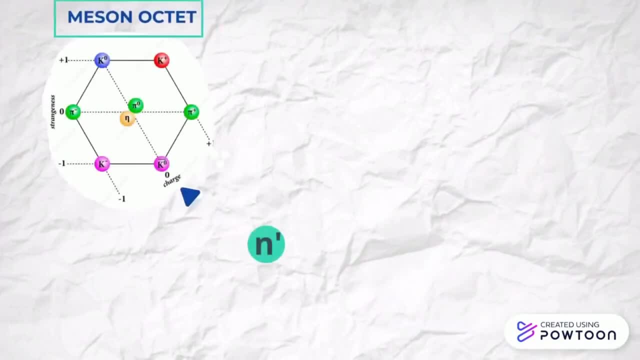 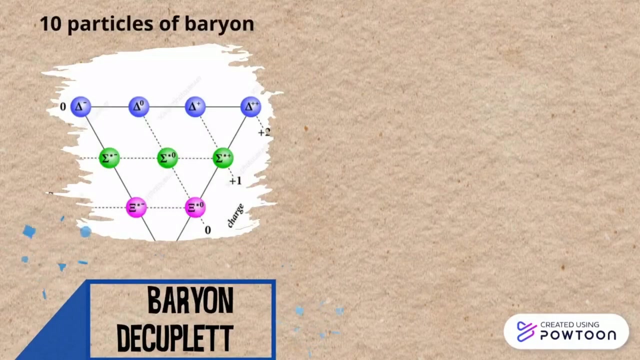 the negative kaon. Later on, eta prime was added into this supermortiflate, and now the supermortiflate is known as mesononate because it consists of nine particles. already The other organization, such as the Baryon Decouplet, which has ten particles of baryon. 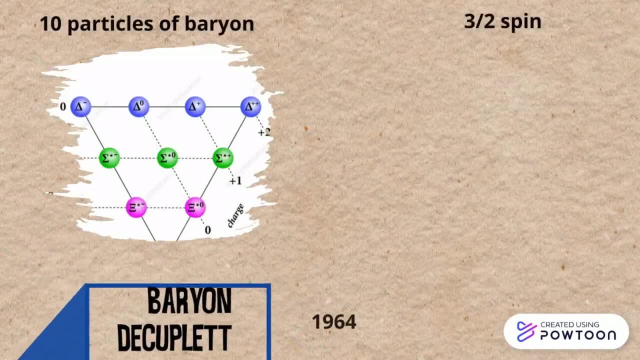 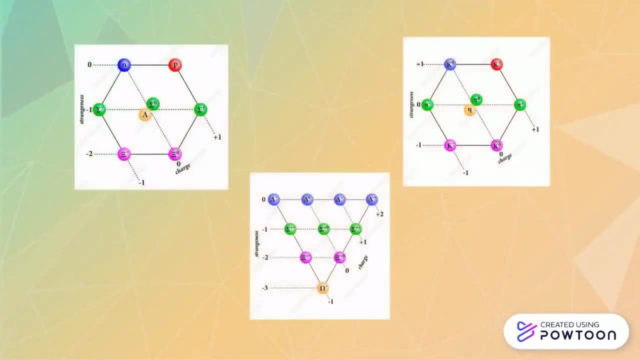 which has the spin of 3 over 2.. In 1964, the negative kaon was discovered and added into this supermortiflate. Note that all of these three supermortiflates have diagonal lines and horizontal lines. The diagonal line represents the strangeness- quantum numbers, while the horizontal line 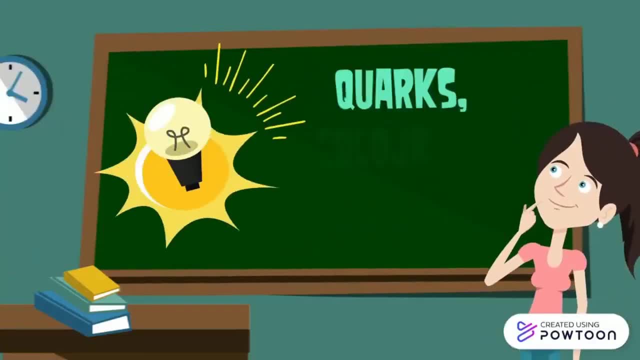 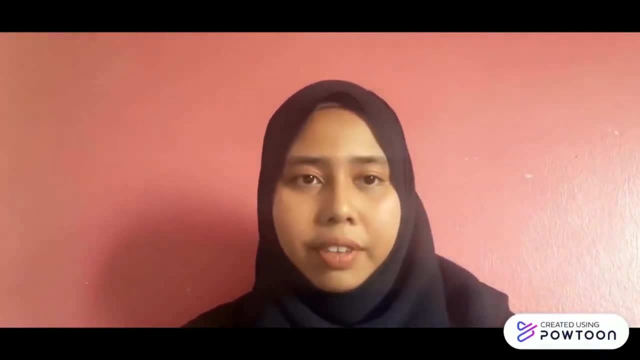 represents the electrical charges. Now I'm going to share with you what is actually quartz, the color and also the flavor of it. Let's see what is the taste of the quartz, since quarks have flavor. Okay, let's see a little history of it. 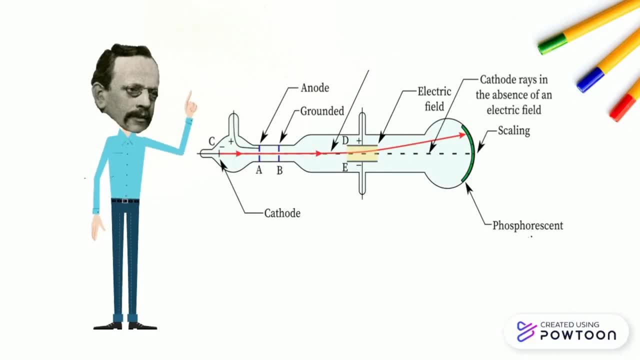 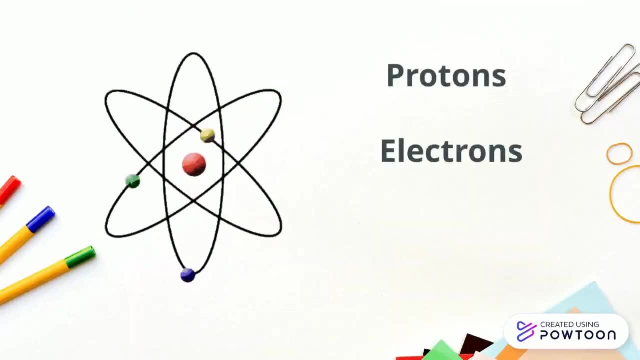 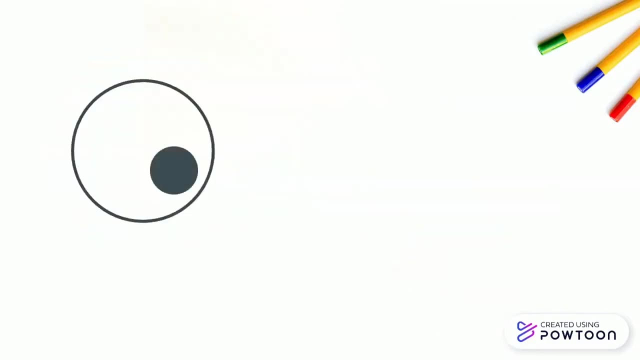 JJ Thomson's experiments with catherine tubes showed that atoms were not the smallest things, And atoms are made of protons, electrons and neutrons. So these three are smallest things? No, Because it is made up of small particles called quarks. 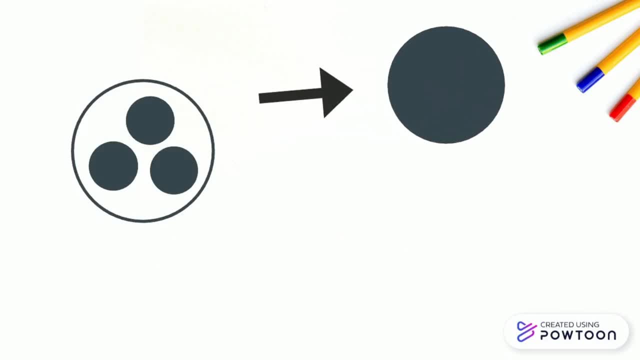 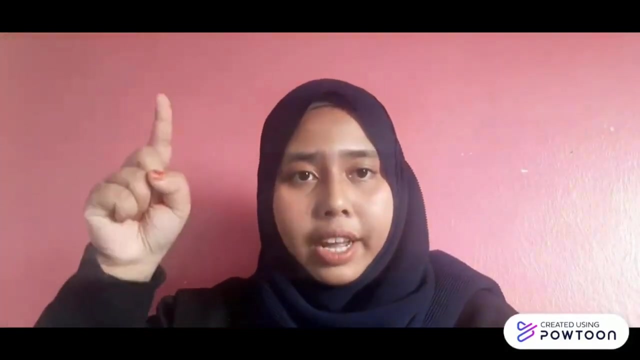 Quarks. It's actually a fundamental constant of matter, which means it doesn't have substructure and cannot be split. And since it cannot be split and broken down into smaller components, quarks known as the smallest things in the universe. Quarks come in three kinds of color charge- red, green and blue, but have nothing to do with the color of visible light or the color of everyday world. 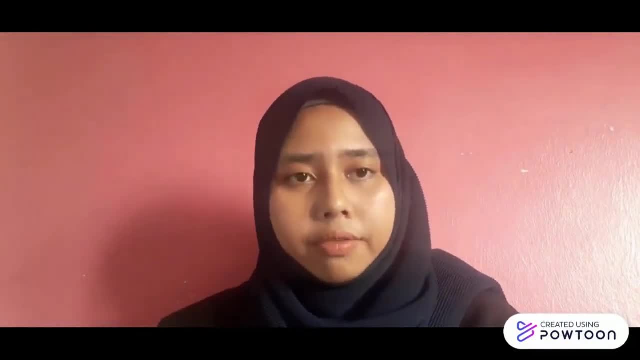 It rather represents a property of quarks that is the source of the strong force. Just as all particles have antiparticles, each color has its own anti-color. The anti-colors are usually referred to as anti-red, anti-green and anti-blue. 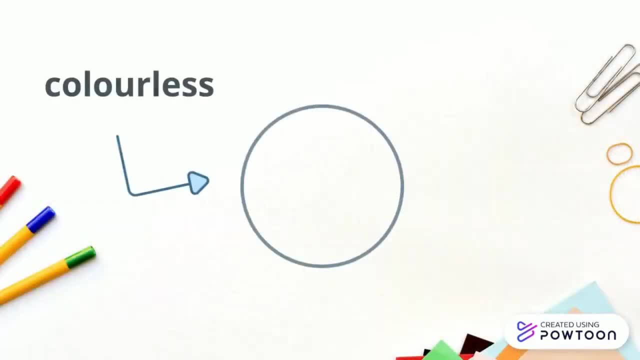 Although quarks have color, the particles they make up are colorless. The red, blue and green quarks present in each particle combine to form a colorless particle and has a zero net color charge. Then how about the flavor of the quarks? 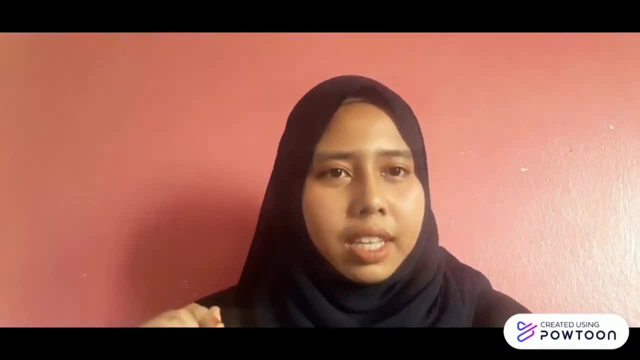 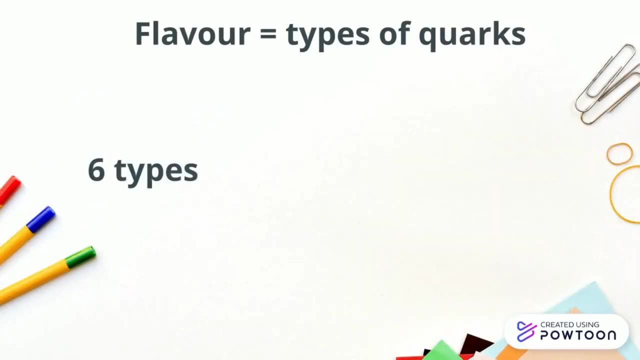 Is it sour, Sweet, Or Maybe it doesn't have any taste at all? Flavor here means the types of quarks. There are six types of quarks that differ from one another in their mass and charge characteristics: Up down, chump, strange bottom and top. 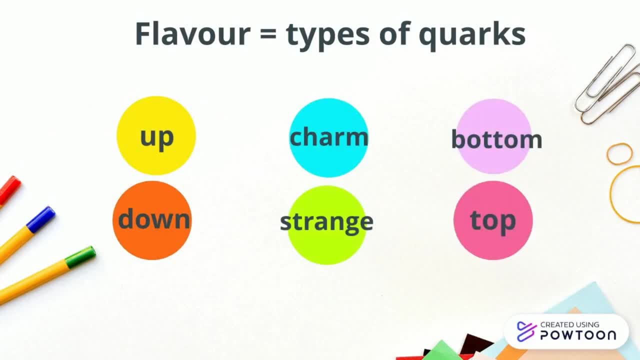 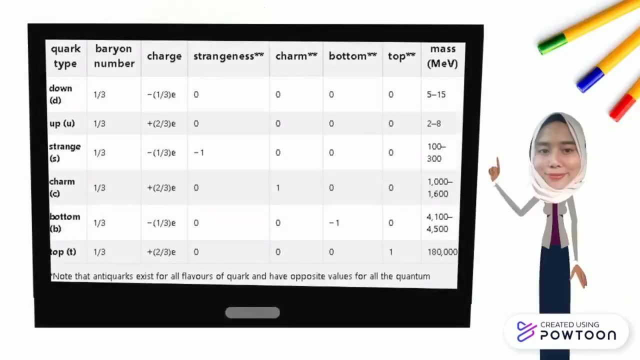 There are three sets of quark pairs and each set of these particles is called a generation. This is the first, second and third. So this is the conclusion of the flavor of the quarks, and one of the important things here is the quark charge. 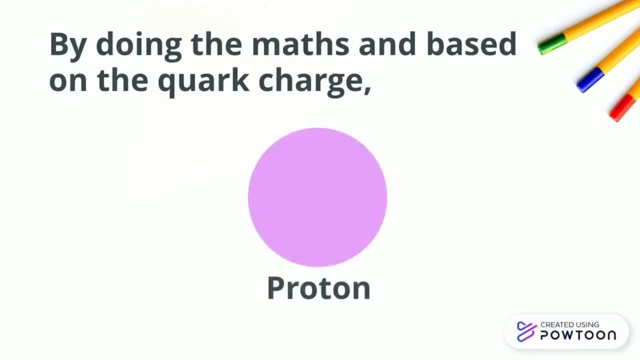 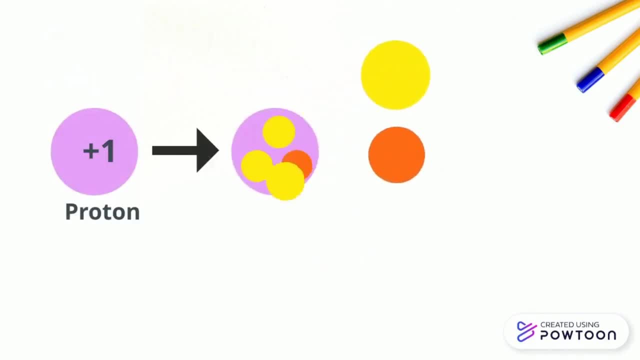 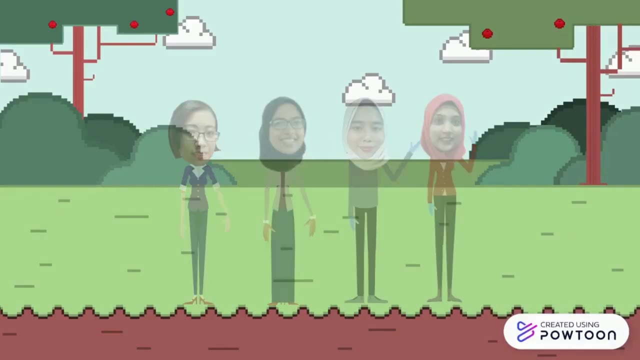 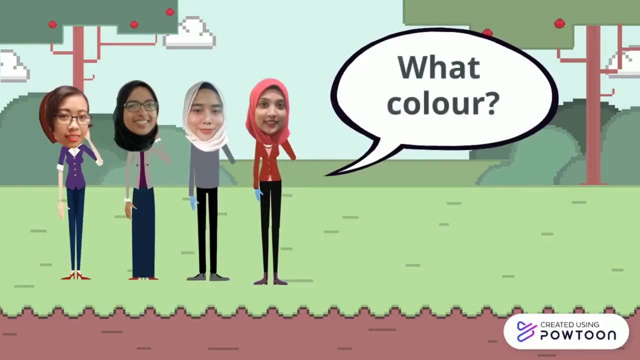 By doing the math and based on the quark charge, we can see how protons have positive charge. To help you remember the quarks color and flavor, let's sing together: Quarks, quarks, what color? what color red do you have? 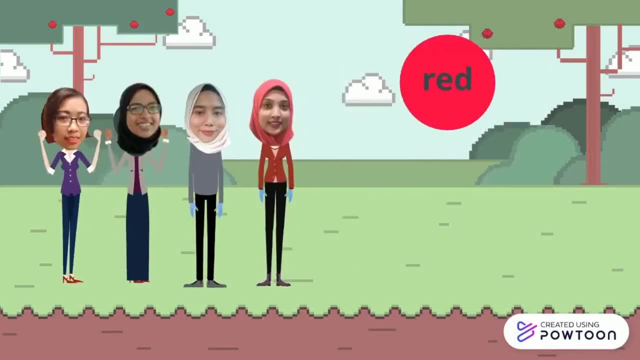 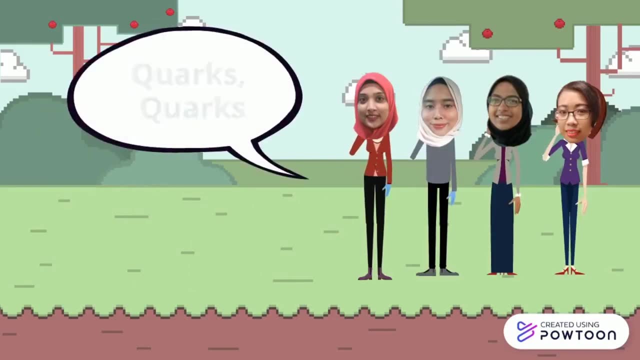 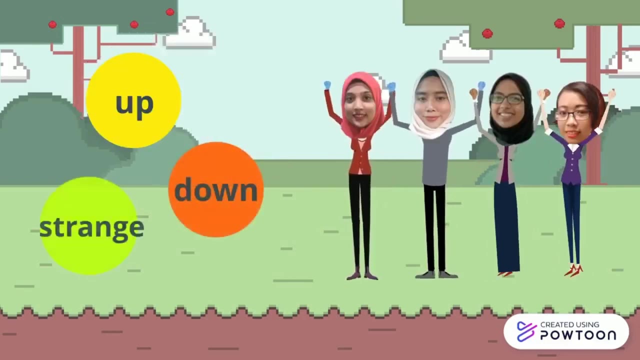 Red, red and red, Red, red and red, Red, red and red, Red, blue and green, Red, blue and green. Quartz, quartz. What flavor? What flavor do you have? Top down, Temp, stretch Some water and pop. 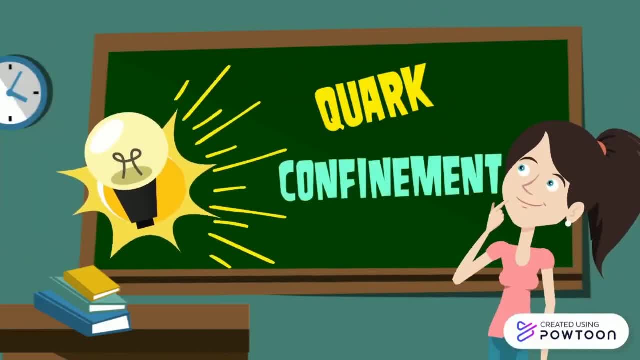 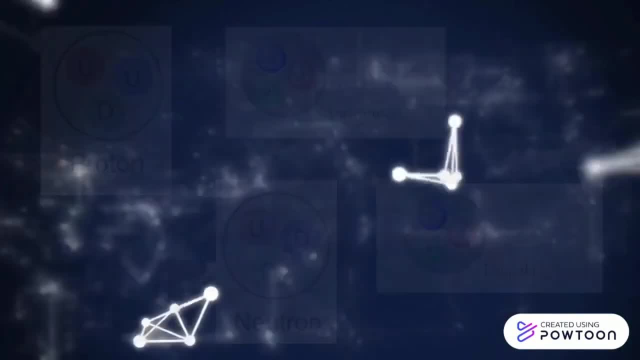 Okay, now I will continue with the final part, which is the core confinement. As my friend mentioned earlier, all of the particles have three quarks inside of them and all of these quarks have strong interaction between them due to the exchange of gluons.